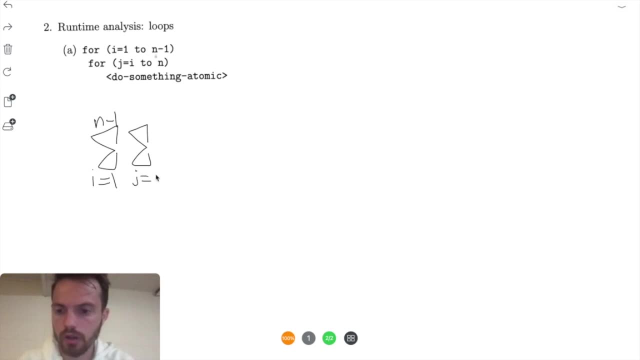 inner loop. the bounds are from j equals i to n, And then here it says: do something atomic Whenever we see that we can just put a plain old one right there. So I think that's parts pretty simple and self-explanatory. 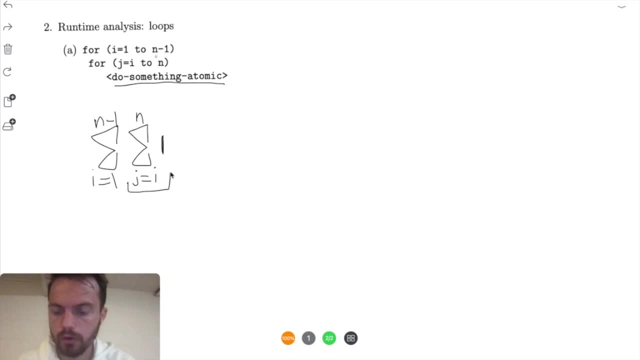 And let's go ahead and deal with this first one here. We always want to work from the right to the left when we do these kind of problems, So we'll start here, on the right. Now we're doing constant: from j equals i to n. Whenever we see that, we know our bounds are from i to n, So we 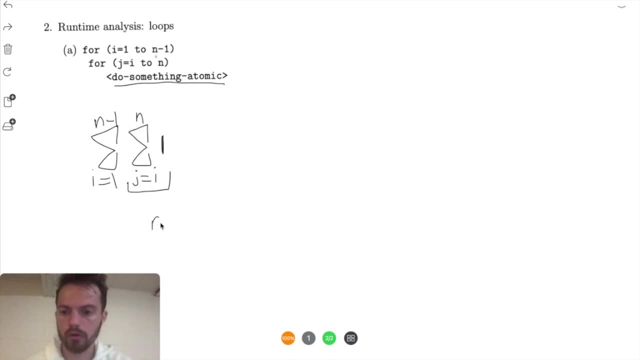 can just use the formula: the second one, second bound, n minus the first bound, i plus one. And one thing that I got tripped on, tripped up on initially was why there's a problem with the plus one here, And the reason for that is, say, we're going from three to five, So we have three. 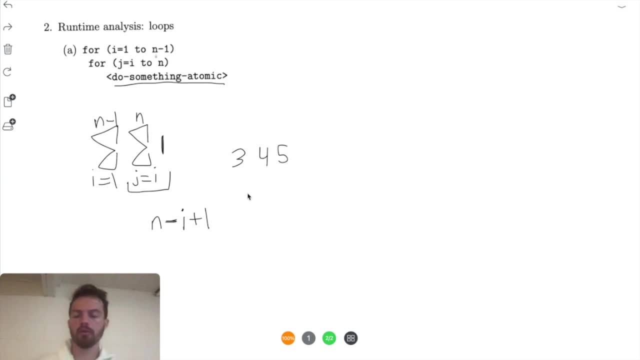 four, five, right here. If we just did five minus three, that would equal two. But we can see here there's obviously not two values, there's three, And that's why you add the plus one, because when you do these bounds there's always an extra one in there. So let's get rid of those now. 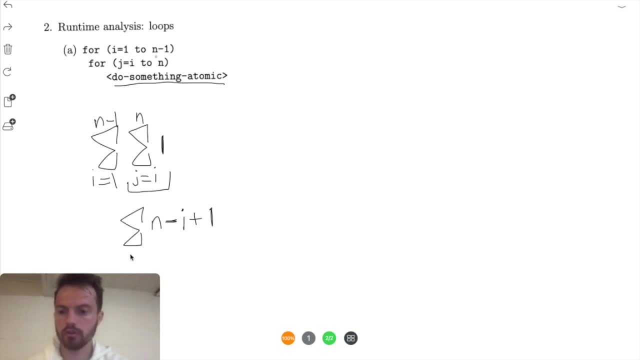 And then we just have to deal with this outer summation. So we have i equals one to n, minus one, And to solve this it'll be easier if we go ahead and split this out into individual summations. So we'll have i equals one. 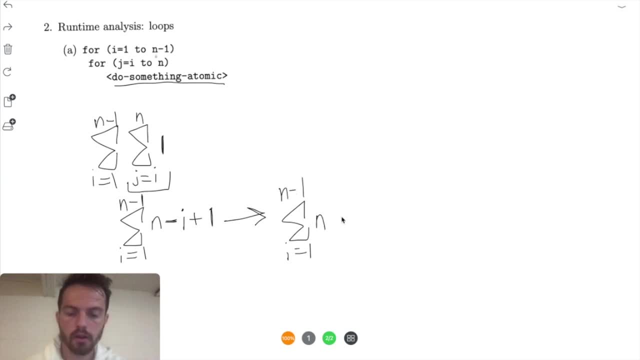 to n minus one. of n minus i equals one to n minus one. of i plus i equals one to n minus one, still of just one. And all we did there was we split up the summation. So first we're going to do the sum of i equals one to n minus one, And then we're going to do the 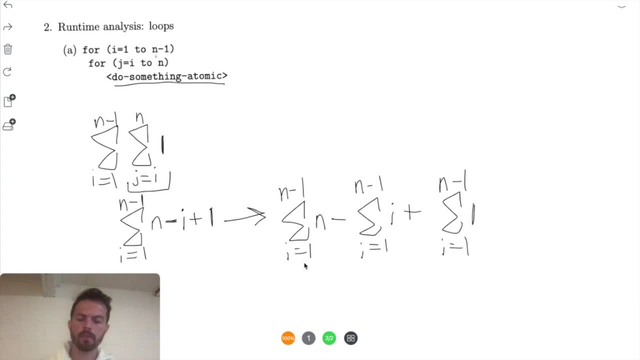 first, There's some tricks here to know. The main ones are: if you see an n, you can just multiply that by the second one up here, And then, if you see an i, there's special formulas you need to know. So first for this n thing, what? like I just said, you can multiply the n minus one. 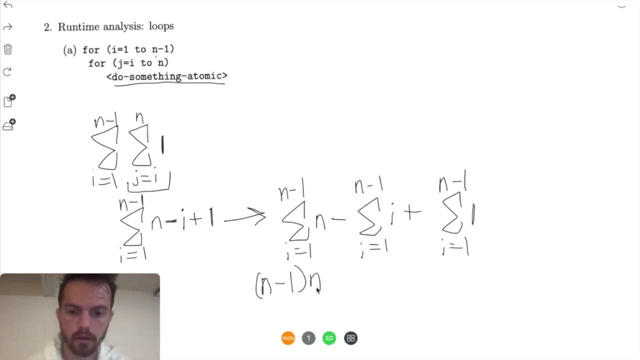 by n, And the reason for that is whatever n is. we're doing that n minus one times. So we're doing n times n times n times n, And we do that from one to n minus one. So since we're doing that n minus one times, we can just do n times n minus one. Then we got to subtract this. 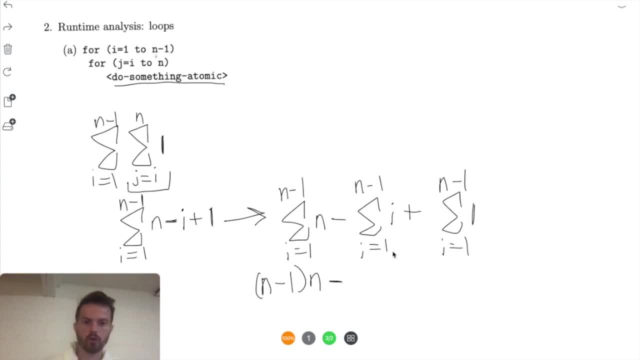 out here. This one has a special formula. when you're going from something to something and there's an i on the right, There's this formula. you need to know which is n, n plus one over two And what this n in here is, whatever your second bound is. So instead of n, we're going to do 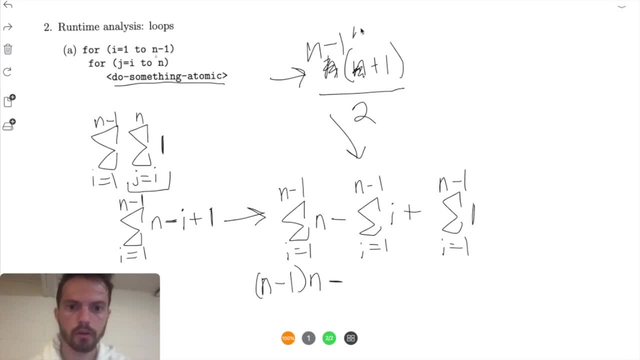 n minus one, n minus one, So we'll make that a little cleaner. down here We're going to have n minus one and then n minus one plus one over two, And there's theoretical ways to go about finding out these summations. I think it's easier. 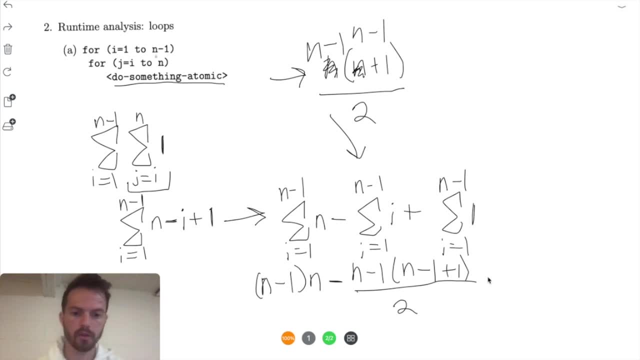 for the purposes of just computer science, trying to get a basic theoretical knowledge, just to memorize these formulas, because there's not that many of them, And then this is just constant right here. So whenever you have content you can use this formula we use back here, which is second bound, n minus one minus. 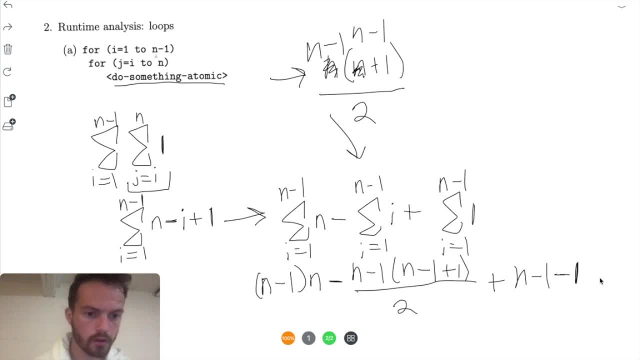 first bound, which is one, and then plus one, So we have a minus one and plus one that cancel out. So we can get rid of that. All right. Then let's just do some simplification here And we're going to get that all equals. 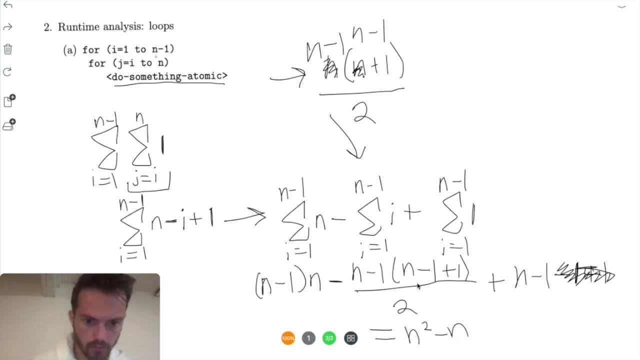 n squared minus n, And then the second part. this here cancels out. So we got minus n squared minus n over two, And then the last part, plus n minus one, Got a minus n and plus n here which we can get rid of, And then we can already.